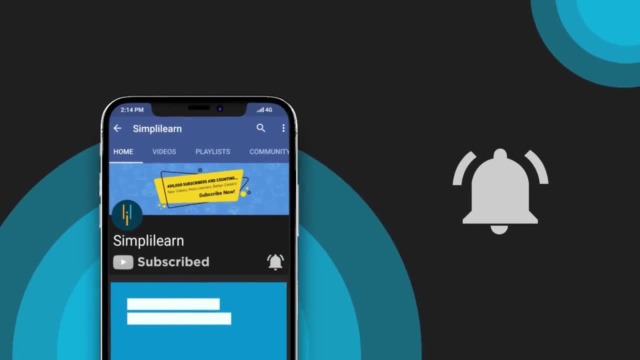 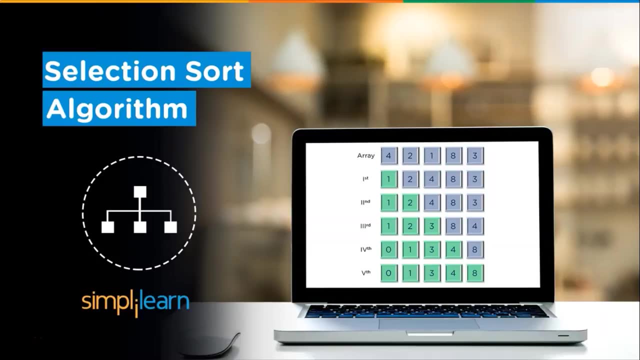 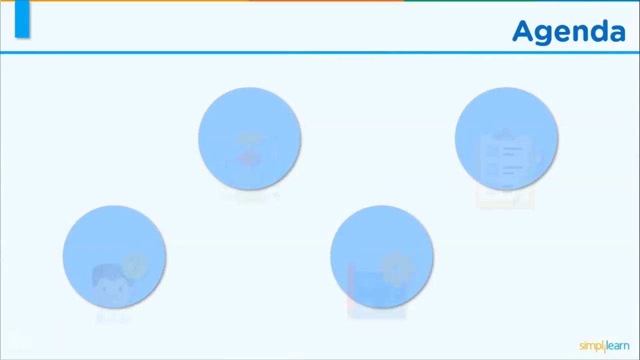 Hey everyone, I am Babakhandelwal and I welcome you all to Simply Learn's YouTube channel. In this session we will discuss Selection Sort Algorithm. We shall begin our session by introducing Selection Sort. Then we will discuss Selection Sort Algorithm After that. 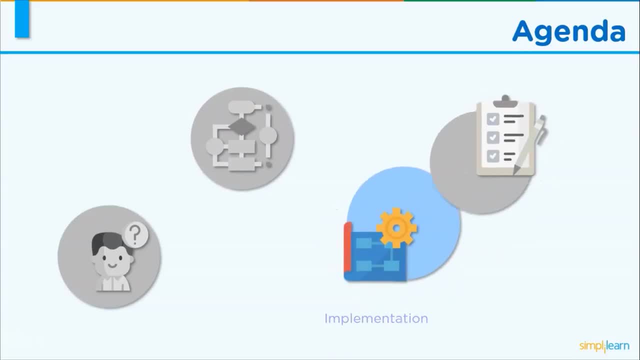 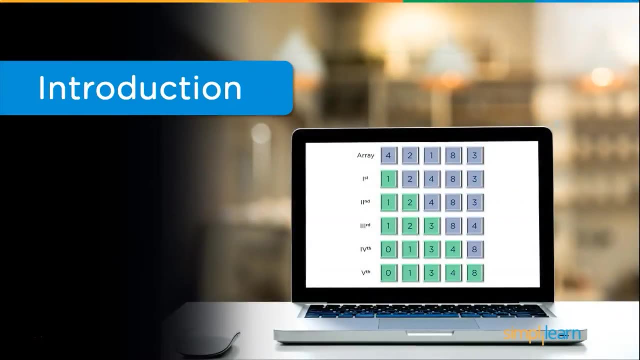 we will implement Selection Sort Algorithm in the Code Editor. Finally, we will sum up what we have learned from this session. Before we begin, make sure you have subscribed to our YouTube channel and clicked on the bell icon below, so you never miss an update. 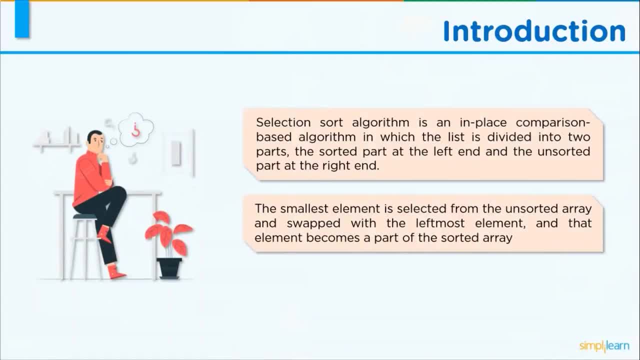 from Simply Learn's YouTube channel. So, without any further ado, let's get started with an introduction to Selection Sort. The Selection Sort Algorithm is an in-place comparison-based method that divides the list into two halves, with the sorted portion on the left and the unsorted half on the right. Then the smallest element from the 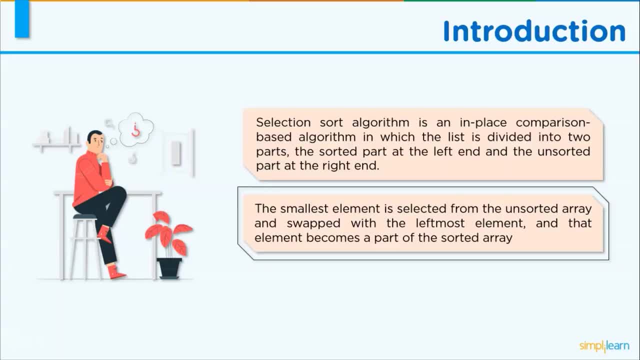 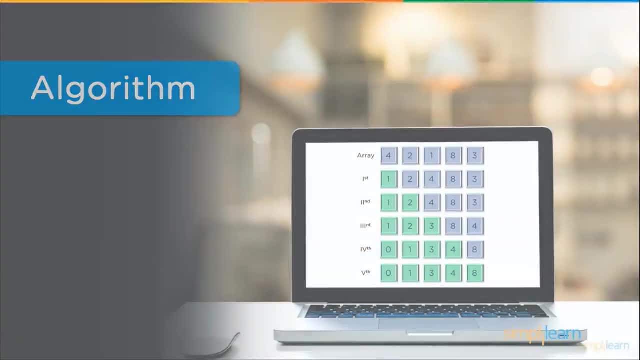 unsorted array is chosen and swapped with the leftmost element, and that element is added to the sorted array. Now let's discuss the Selection Sort Algorithm. Let's say we have an array. First we will divide this array into two sub-arrays, unsorted. 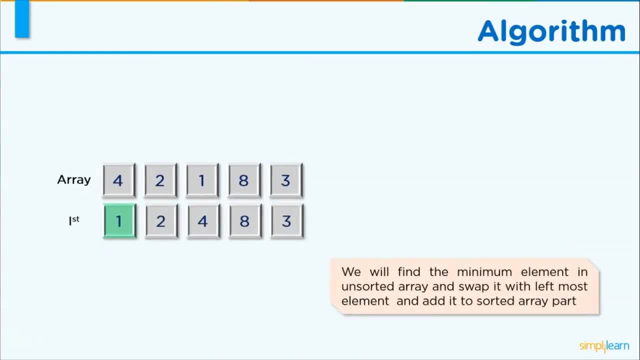 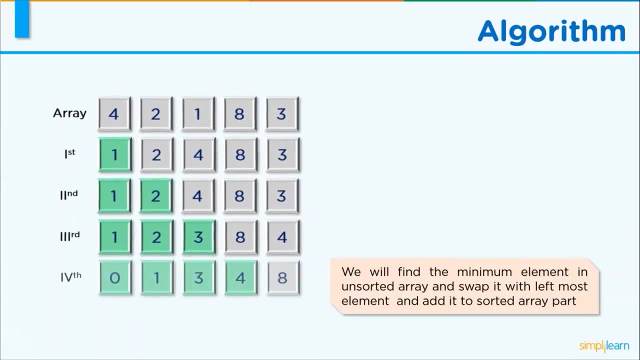 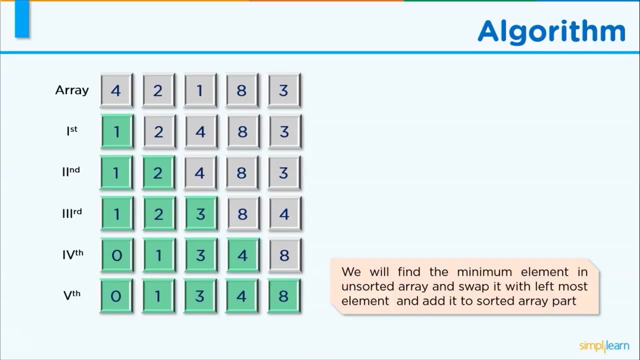 array and sorted array. Then we will divide the minimum element from the unsorted array and swap it with the leftmost element of this unsorted array. After that we will add it to the sorted array. We will keep repeating this process until there are no elements. 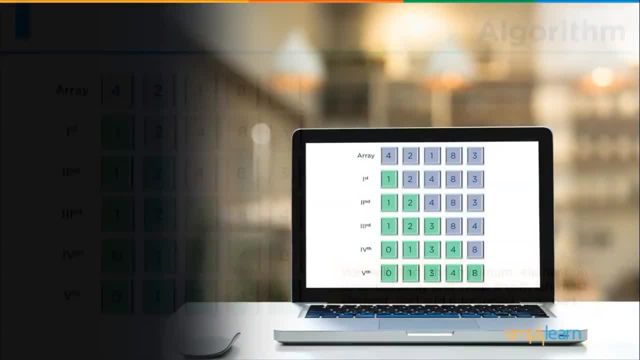 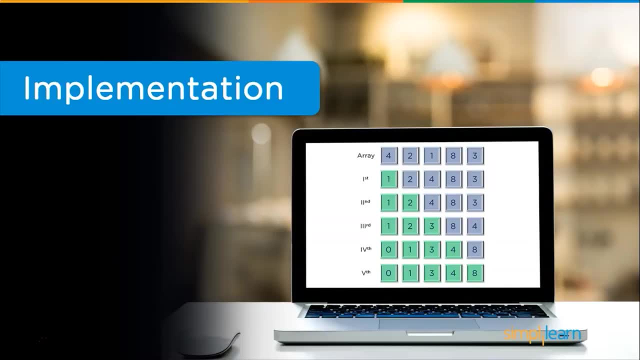 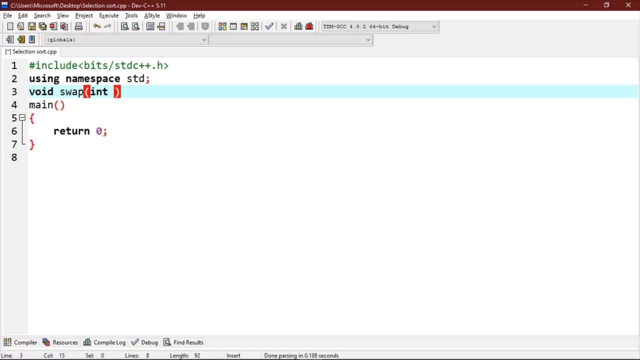 left on the unsorted array. We have now introduced Selection, Sort and its algorithm. Now let's implement this algorithm in the code editor. We will start by creating a function, SWARQ. The argument will be: integer pointer x. comma integer pointer y. comma integer pointer x. 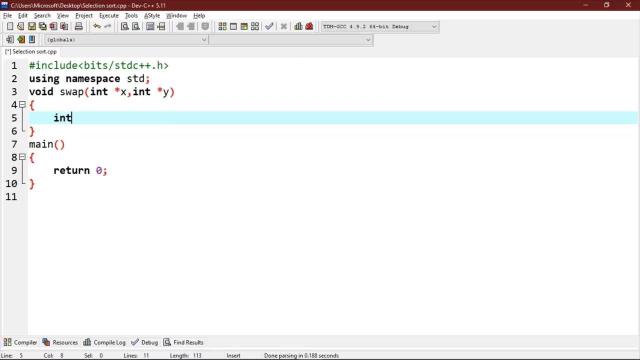 We will declare an element, temp, to store the value of pointer x, Then we will store pointer y's value in x, Then we will store temp's value in y, And that's how we can swap them. Next we will write the definition of Selection: Sort, function, void, selection, sort. 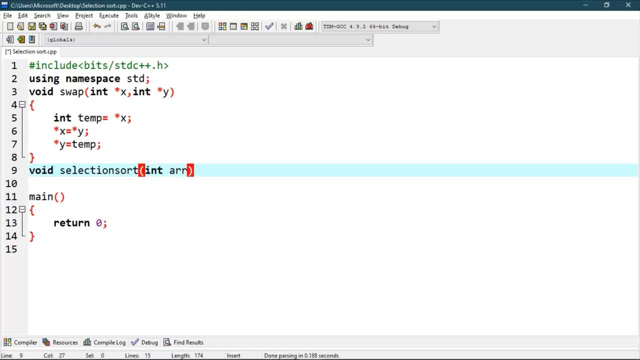 The argument will be int array, arr, comma, int n. We will declare variables int i, j, 0, over right and symbol. Then we will use integer pointer n to initializeấp argument. This argument will be Java pack question. 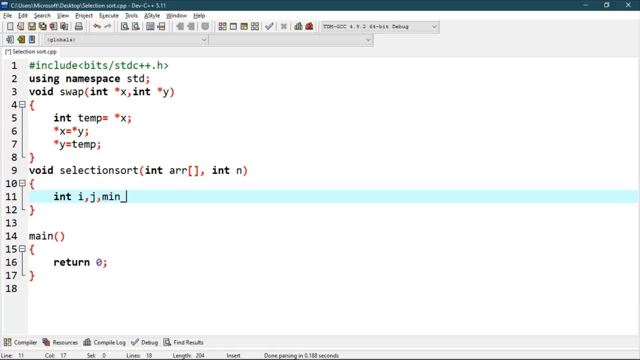 Next we will write the definition of Selection, Sort function, void, selection, sort. Then we j and a min underscore, idx variable to store the minimum index. Now we will one by one move boundaries of unsorted subarrays. So for loop, i is equal to 0, where i is less than n-1, i++, we will find the minimum element. 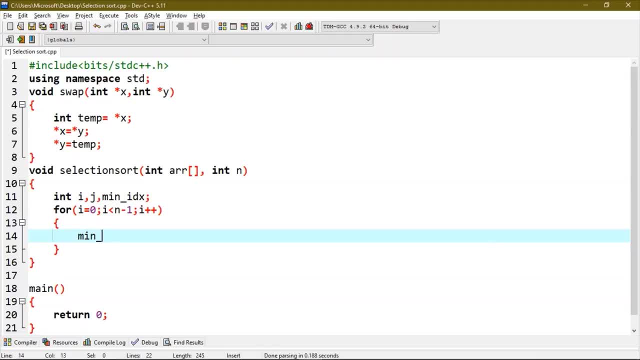 in this unsorted array. so min underscore idx is equal to i. Now for j is equal to i plus 1,. j less than n, j++. if array element at jth location is less than array, If array at the min index, then min idx will be updated with j. 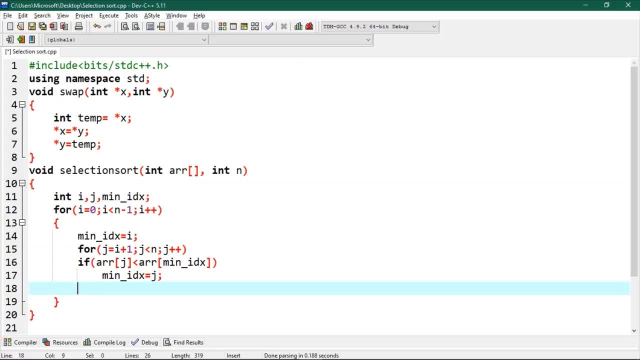 Now we will swap the found minimum element with the first element. so we will call swap function with the argument as: m%arr at min idx, m%arr at jth location. Now we will write a function to print this array, So void. 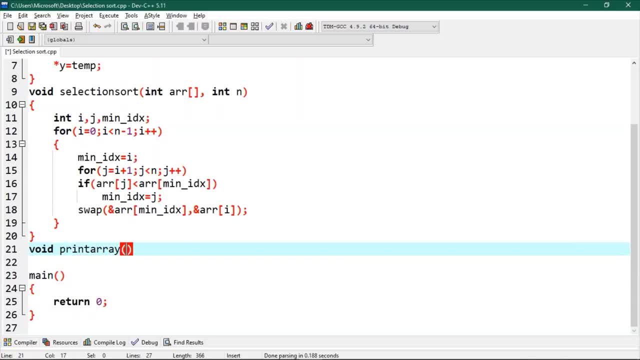 int array argument. as int arr and its size, int n, for loop, int i is equal to 0, i less than i plus plus t out, arr at i t out, And now the error will be added to give working result. 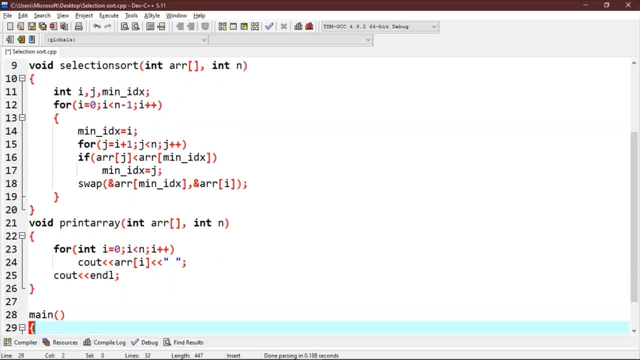 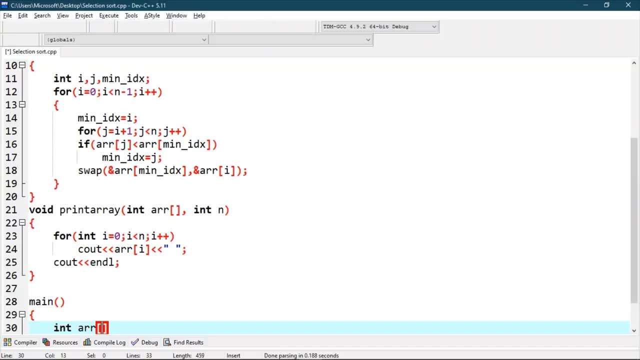 Enter Now. str zweiten feels like vk opens up And נ one thing: i is not inside correct. Now we will write the code for the main block. so int arr is equals to 4 comma 2 comma 1. 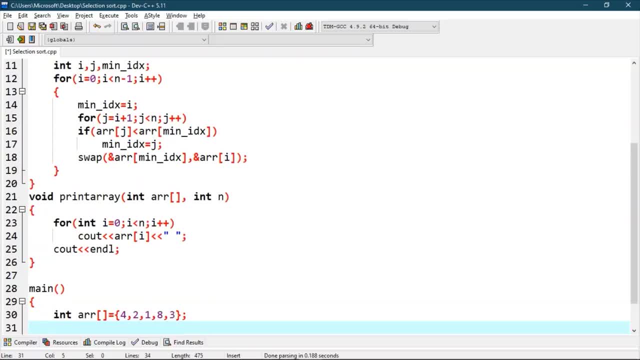 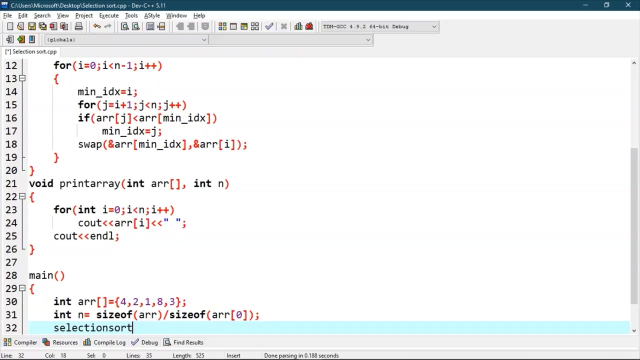 comma 8, comma 3, we will find the size of this array, so int n is equals to size of array arr divided by size of this array's first element. Now we will call selection sort function argument as arr. comma n. then we will try to print this: